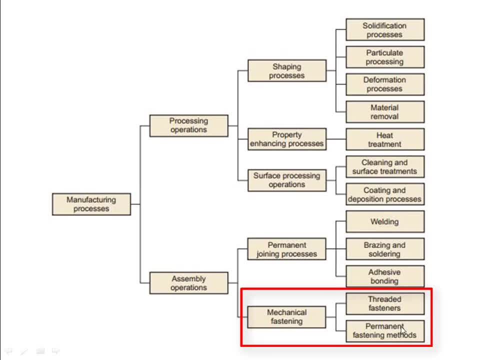 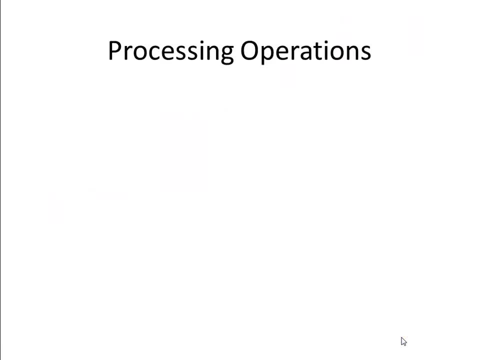 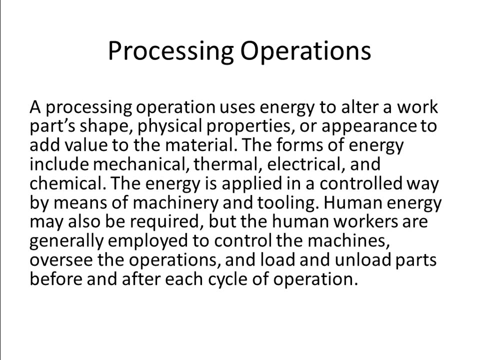 And mechanical fastening is two types, that is, threaded fasteners and permanent fastening methods. So let's discuss one by one, Processing operations. Processing operation- usually Processing operation- uses energy to alter a work part, shape, physical properties or appearance, to add value to the material. 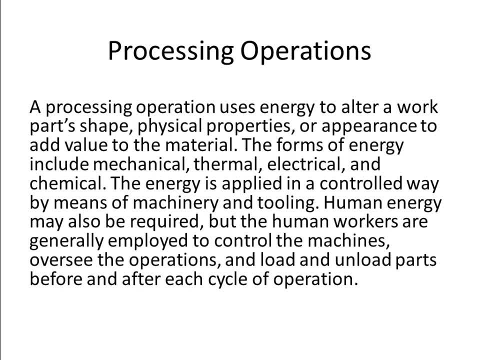 The form of energy includes mechanical, thermal, electrical and chemical. The energy is applied in a controlled way by means of machinery and tooling. Human energy may also be required, but the human workers are generally employed to control the machines, oversee the operations and load and unload parts before and after each cycle of operation. 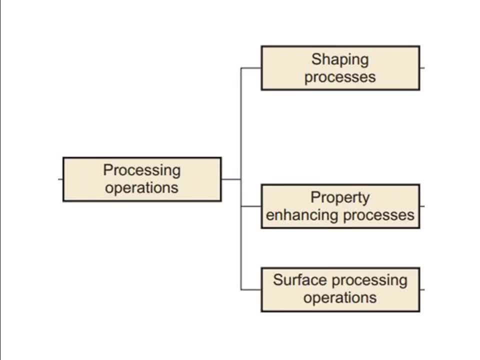 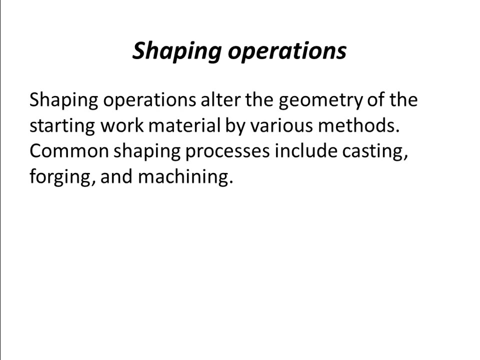 Processing operations is divided into three parts, as we discussed earlier: Shaping processes, property enhancing processes and surface processing operations. Shaping operations- Shaping operations alter the geometry of the starting work material by various methods. Common shaping processes include Casting, forging and machining. 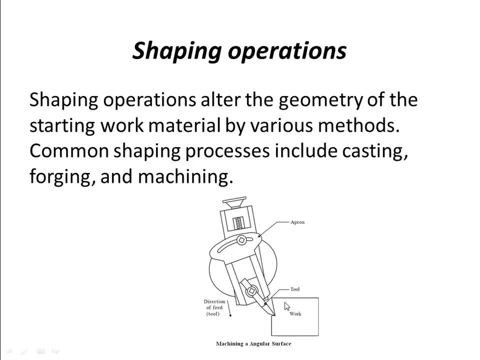 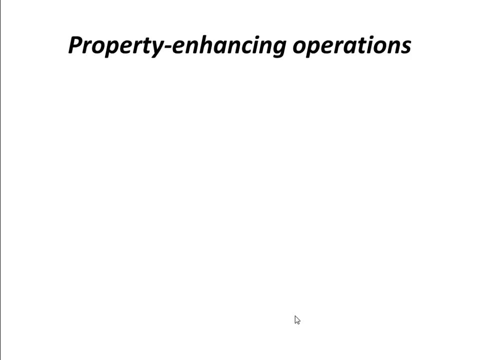 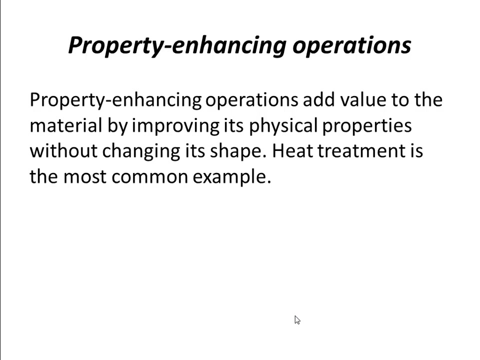 And there is an example. This is the work and this is the machine tool. So machine tool is used to give geometry or to change the geometry of the work piece by machining And property enhancing operations. Property enhancing operations add value to the material by improving its physical properties. 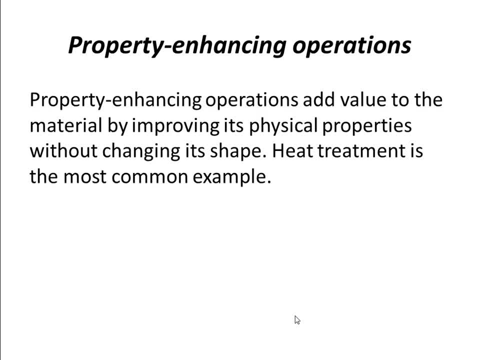 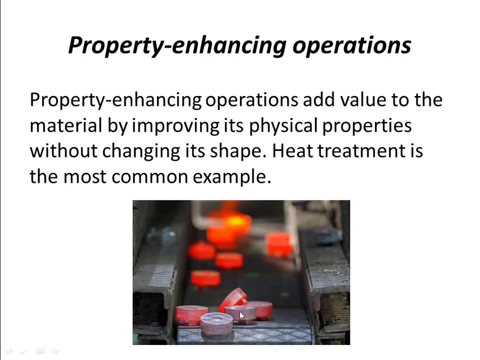 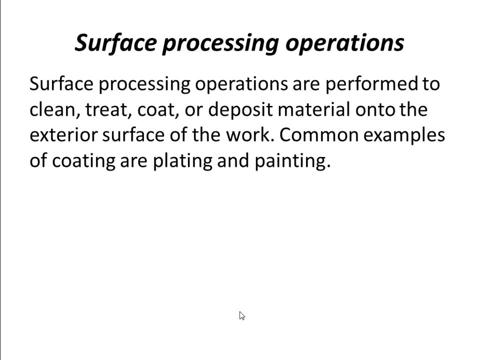 Without changing its shape. Heat treatment is the most common example, And as an example, These objects are heated to enhance the property. Then surface processing operations: Surface processing operations are performed to clean, treat, coat or deposit material onto the exterior surface of the work. 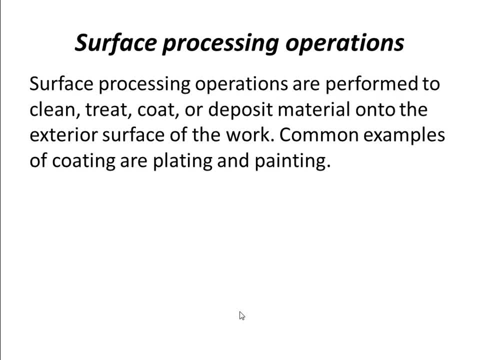 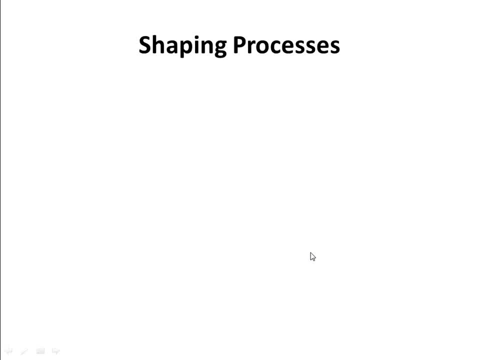 Common examples of coating are plating and painting, And there is an example of painting Shaping processes. Most shape processing operations apply heat, mechanical force or a combination of these two effects, A change in geometry of the work material, And there is an example. 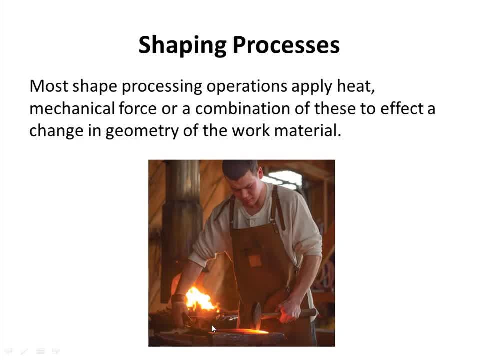 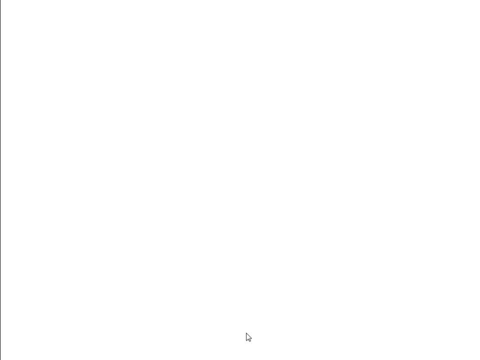 Which is being heated and then applying heat, Mechanical force is applied to give a defined shape. Shaping process is divided into four categories And we have already discussed these four And let's discuss one by one. First one is solidification process. 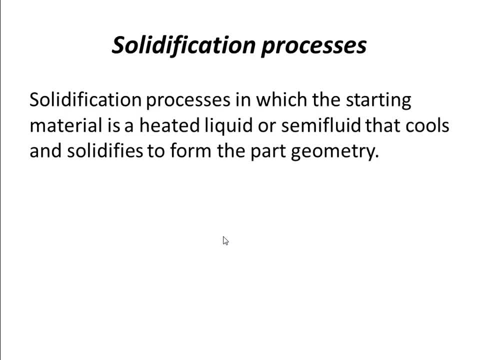 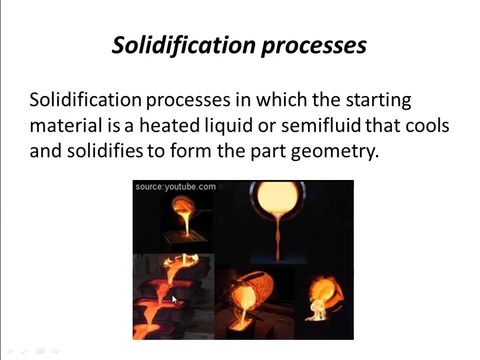 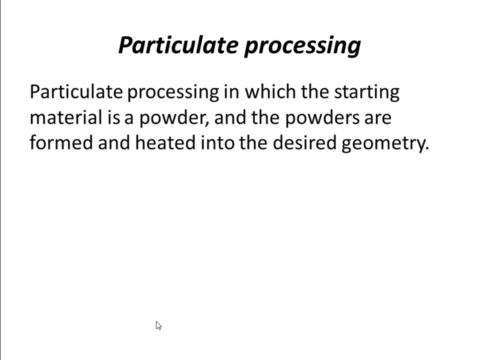 Solidification process in which the starting material is a heated liquid or semi-fluid That cools and solidifies to form the part geometry And as an example, This is liquid and this liquid are poured and then cooled to give a desired shape, Then particular processing. 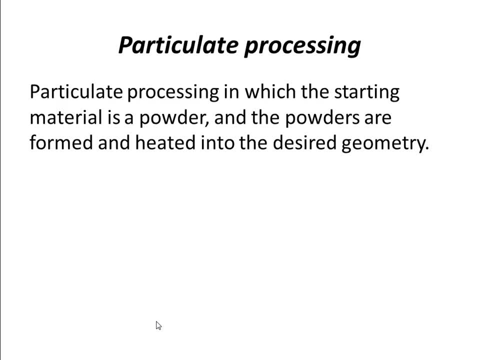 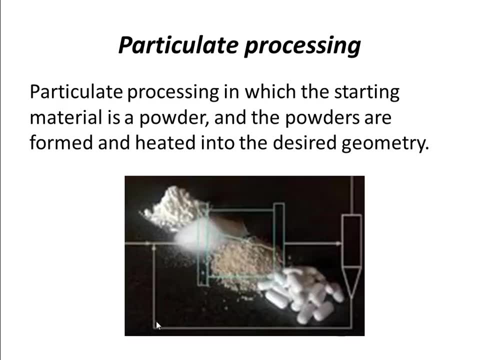 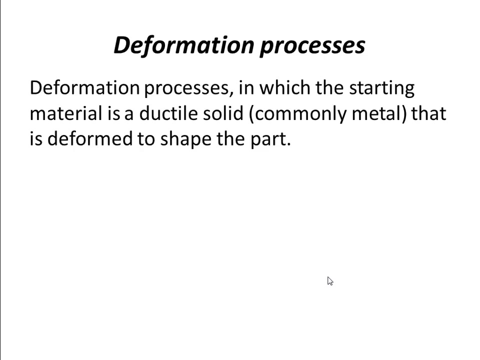 Particular processing, in which the starting material is a powder And the powders are formed and heated into the desired geometry. And there are three types of powders And using these powders, Desired shape have been found. Now deformation processes: Deformation processes in which the starting material is a ductile solid. 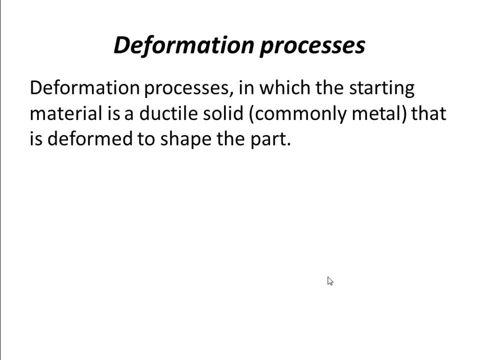 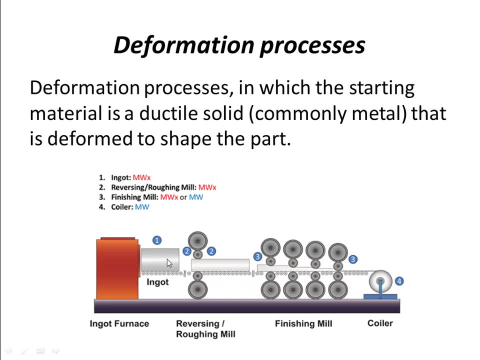 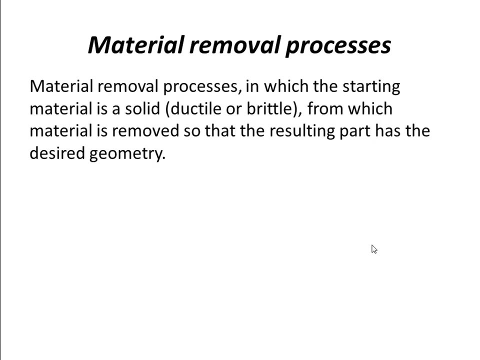 Commonly metal That is deformed to shape the part And there is a ductile material Which is rolled to match the sheet metal. Then material removal processes. Material removal processes in which the starting material is a solid That can be brittle or ductile. 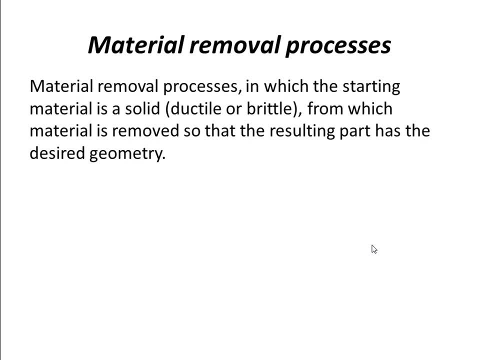 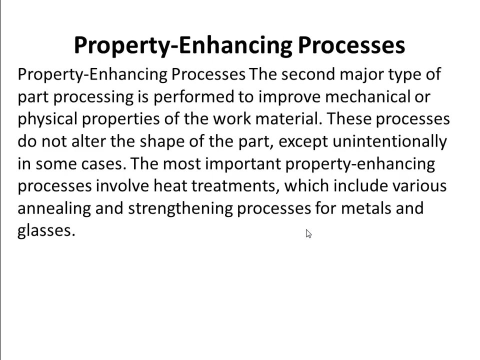 From which material is removed So that the resulting part has the desired geometry, And we know this one. So from this part the material is removed to give this desired shape. Property enhancing processes. Property enhancing processes- the second major type of part processing- is performed to improve mechanical or physical properties of the work material. 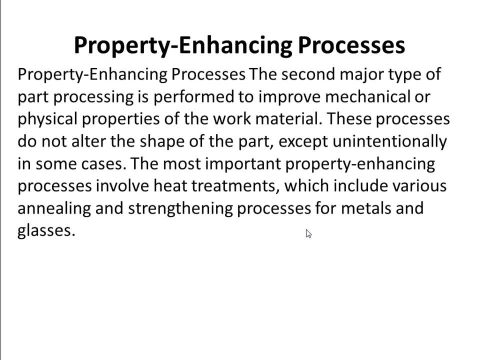 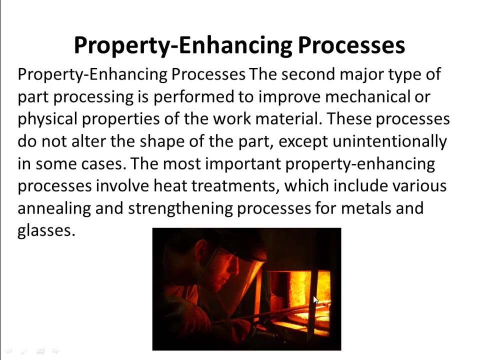 These processes do not alter the shape of the part, except unintentionally in some cases. The most important property enhancing processes involve heat treatment, Which include various annealing and strengthening processes for metals and glasses, And there is an example of heat treatment. So surface processing operations are two types. 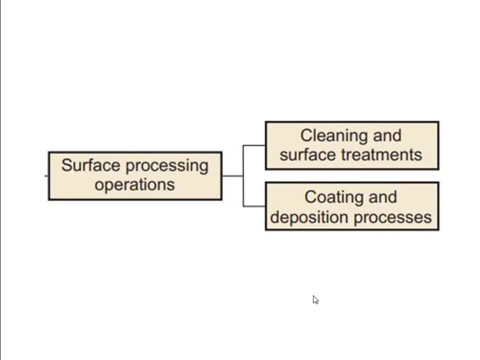 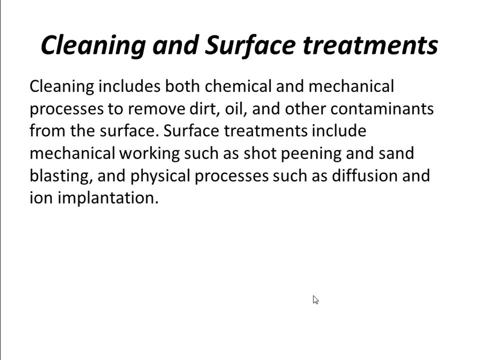 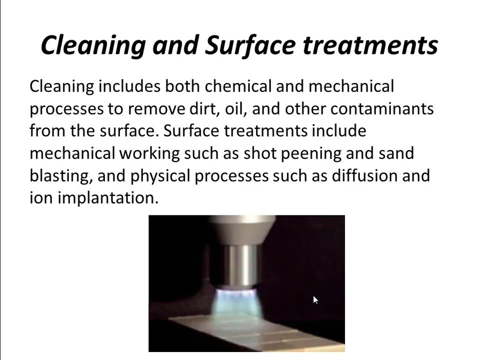 Cleaning and surface treatments, and coating and deposition processes. Cleaning and surface treatments. Cleaning includes both chemical and mechanical processes To remove dirt oil and other contaminants from the surface. Surface treatments include mechanical work such as shot pinning and sandblasting, And physical processes such as diffusion and ion implantation. 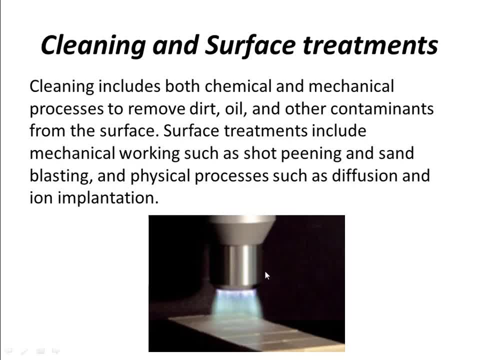 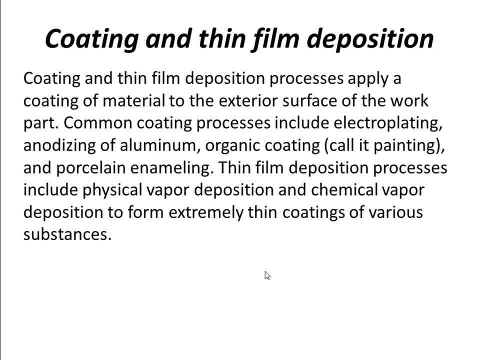 And there is an example of surface treatment: Coating and thin film deposition. Coating and thin film deposition processes apply a coating of material to the exterior surface of the work. Common coating processes include electroplating, anodizing of aluminum, organic coating and porcelain annealing. 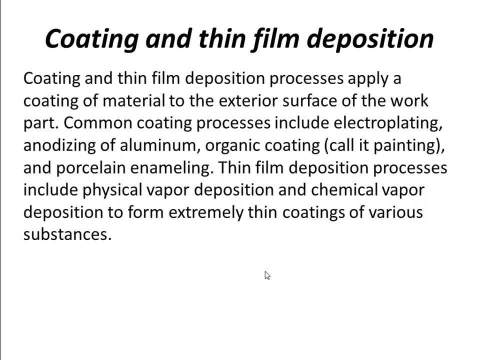 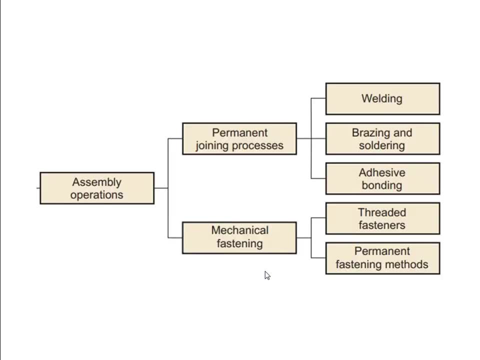 Thin film deposition processes include physical vapor deposition and chemical vapor deposition To form extremely thin coatings of various substances. And there is an example of thin film deposition Coating and thin film deposition Now assembly operations. That is initially two types, That is, permanent joining processes and mechanical fastening. 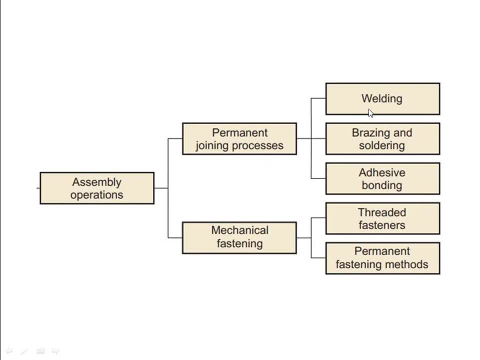 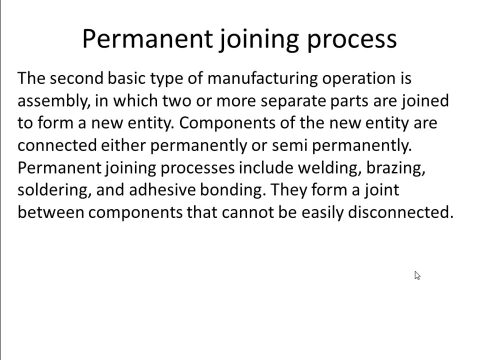 Then permanent joining processes- Welding, brazing, soldering and adhesive bonding- Then mechanical fasteners, threaded fasteners and permanent fastening methods. Let's discuss about permanent joining processes. The second basic type of manufacturing operation is assembly In which two or more separate parts are joined to form a new entity. 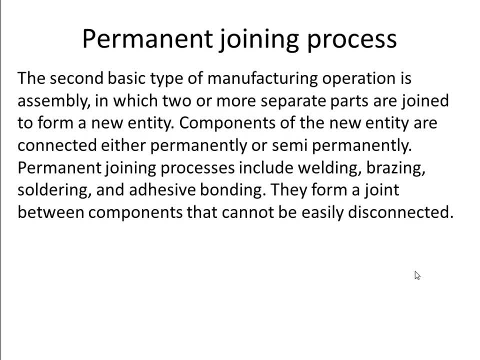 Components of the new entity are connected either permanently or semi-permanently. Permanent joining processes include welding, brazing, soldering and adhesive bonding. They form a joint between components that cannot be easily disconnected, And there is an example of welding, That is gas welding. 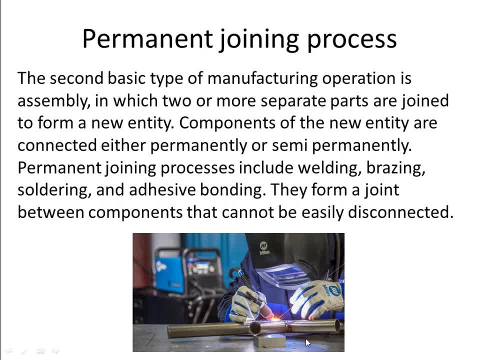 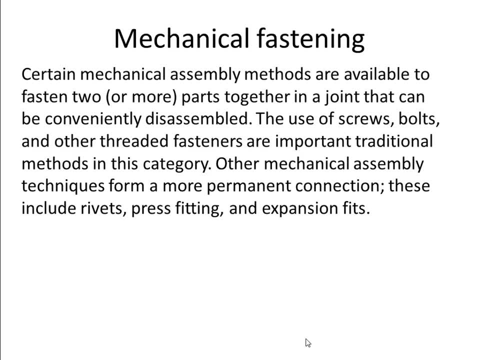 And by this gas welding these pipes are joined permanently. Mechanical Fastening: Certain mechanical assembly methods are available to fasten two or more parts together in a joint that can be conventionally disassembled. The use of screws, bolts and other threaded fasteners are important traditional methods in this category. 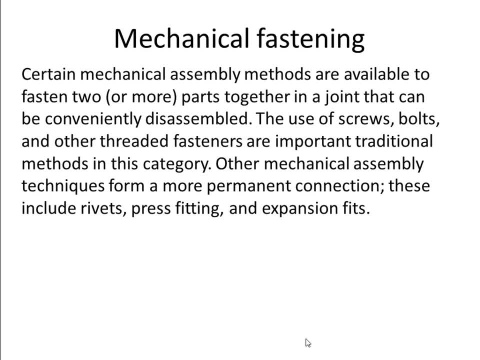 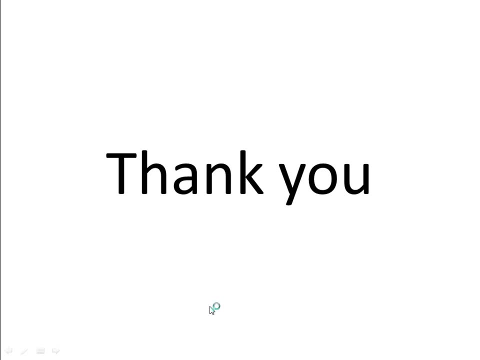 Other mechanical assembly techniques form A more permanent connection. These include rivets, press fitting and expansion fits, And there are three examples of mechanical fastening. And thank you for being with me. 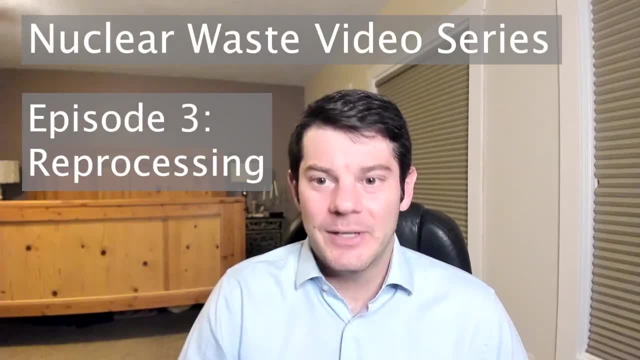 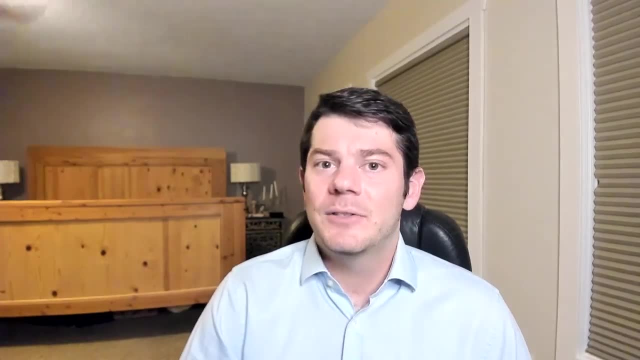 Hello everyone and welcome back to the nuclear waste video series. Today we are going to discuss reprocessing, which is perhaps my personal favorite approach for disposing of nuclear waste. Let's start our discussion today by asking what if we could recycle our nuclear waste just like how I recycle my jokes? 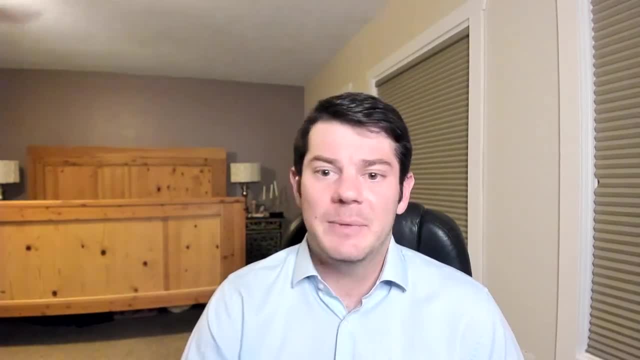 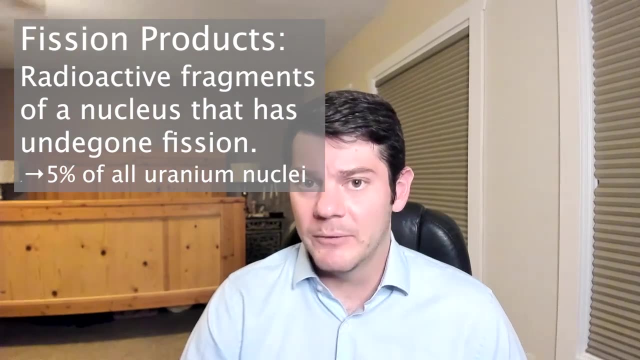 As I discussed in the first video, nuclear waste is radioactive because it contains radioactive fission products. However, only about 5% of uranium atoms in spent nuclear fuel have undergone fission. The rest is perfectly good uranium. So instead of burying this spent nuclear fuel underground, 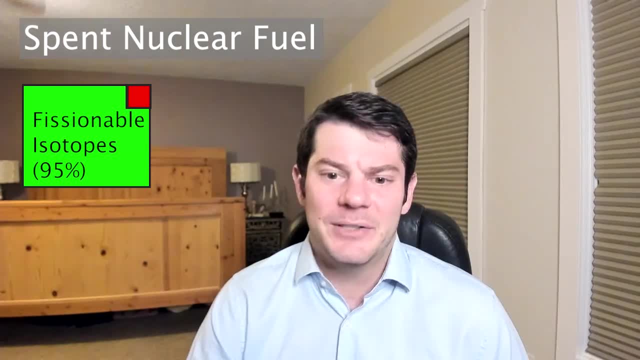 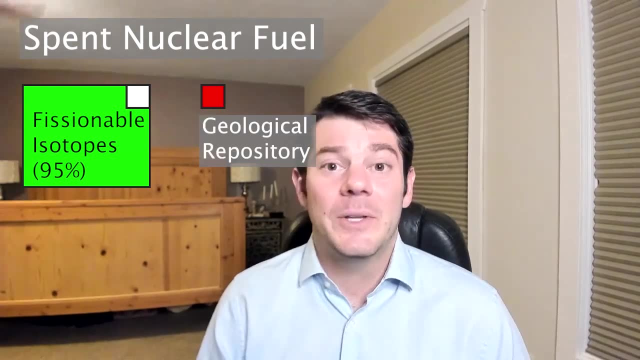 in a geological repository and throwing away 95% of our uranium. what if we could separate out those nasty radioactive fission products and just bury them instead? After we dispose of those radioactive fission products, we could then recycle the fissionable nuclei by putting them back into. 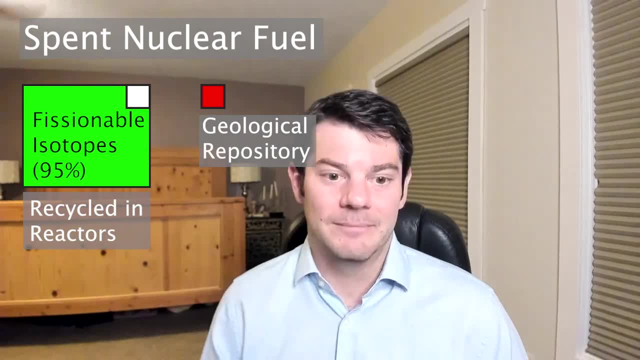 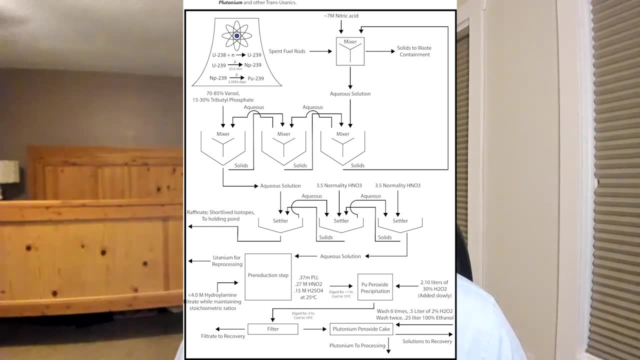 a nuclear reactor, thus generating even more energy. Reprocessing does just this. Through chemical processes such as the purix or uric process, we can dissolve spent nuclear fuel and then chemically separate out different nuclides in the fuel. This is great. Heavy actinides such as plutonium and americium and curium can all undergo fission, as can the leftover uranium under certain conditions. So if you reprocess the fuel and take these fissionable nuclides and put them back into a nuclear reactor, then, bam, you have more fission fuel and basically unlimited power.